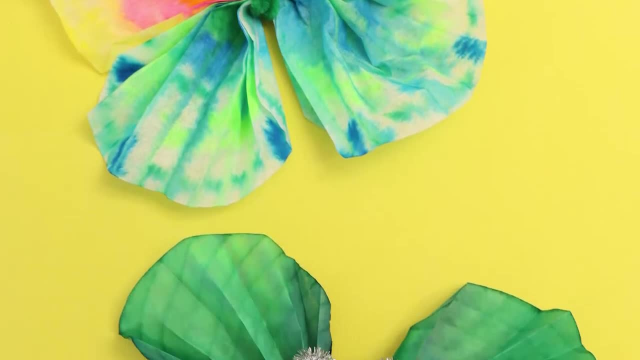 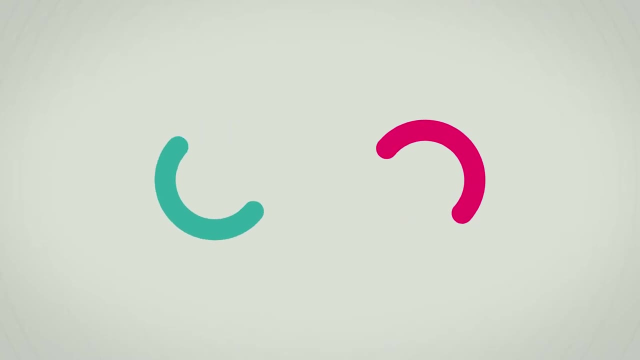 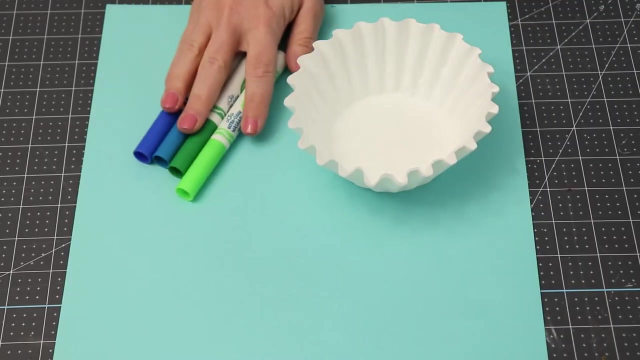 This butterfly craft is perfect for spring: Simple supplies, easy to make. this is great for kids and fun for adults. Here's what you need: Start with two coffee filters per butterfly, some washable markers, a pipe cleaner and a little spray bottle of water. This is the 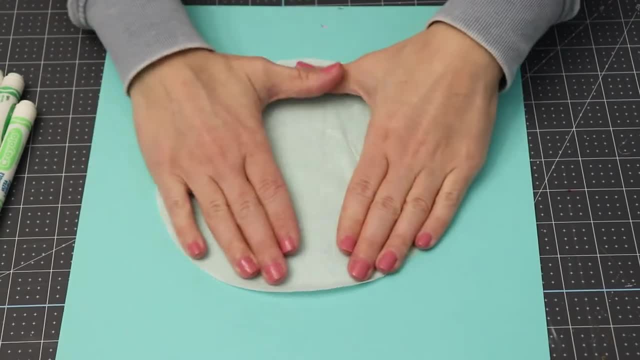 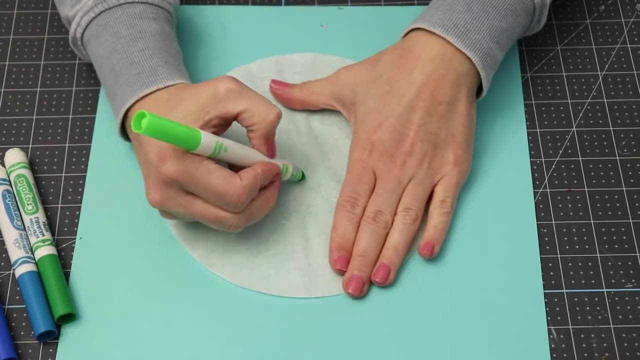 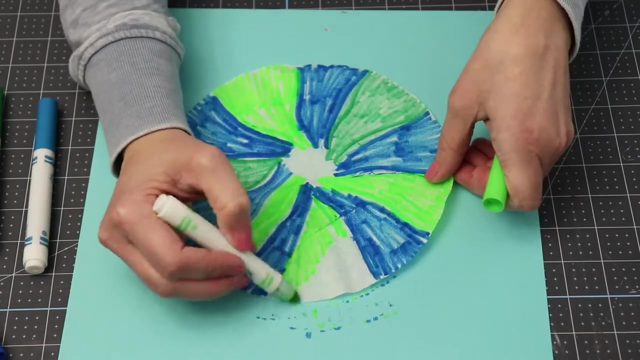 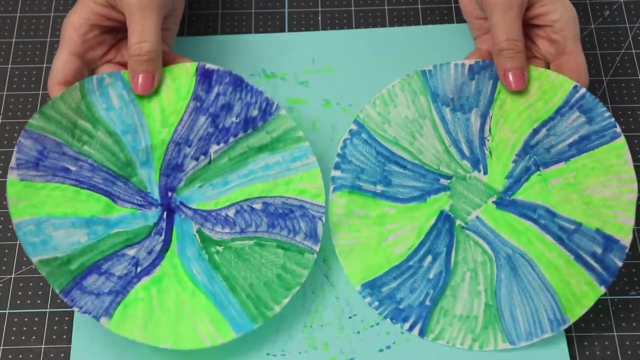 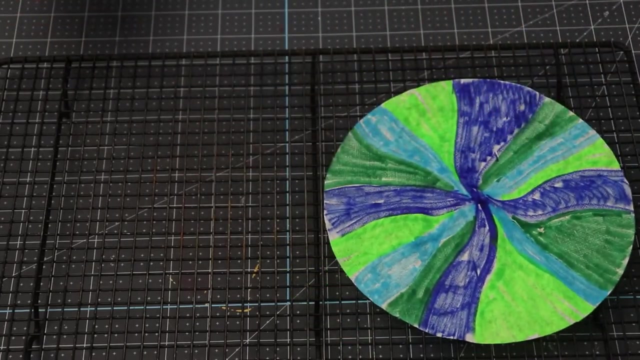 fun part. Open up a coffee filter and start coloring You want your coloring to touch. Ideally, these colors are gonna blend together. at the end here With two coffee filters fully colored in, place them on a metal drying rack like I have here, or in a metal pan. Then grab your little spray bottle of water and 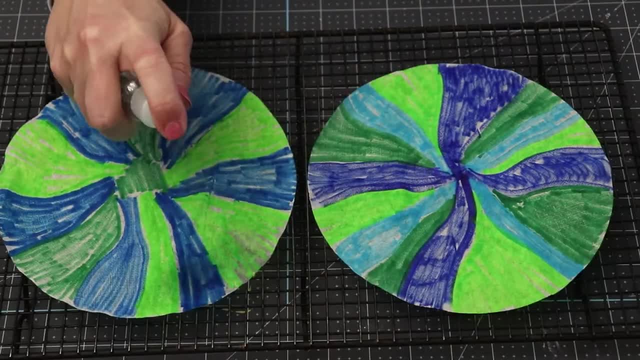 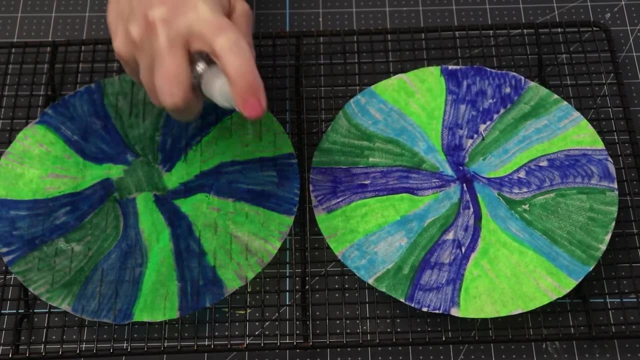 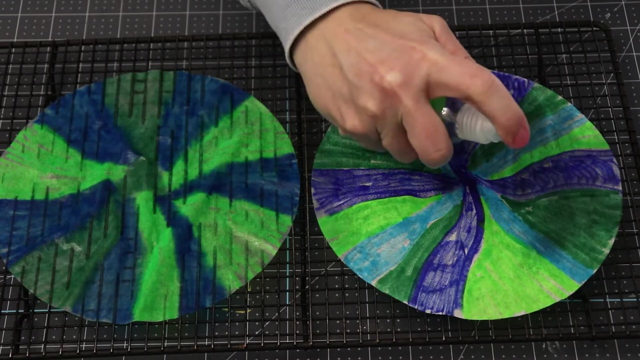 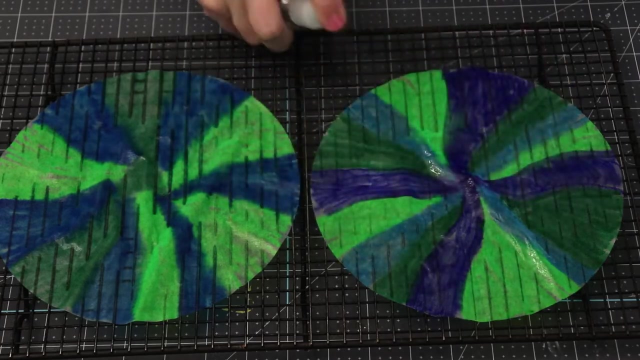 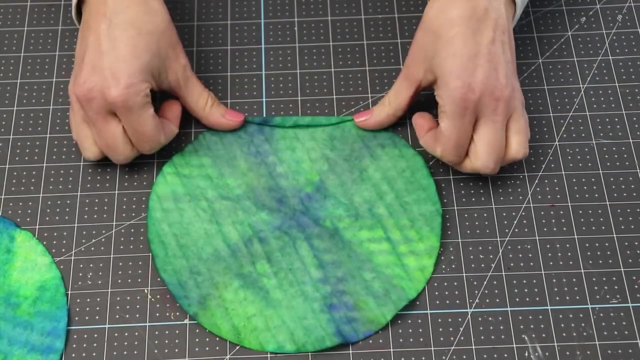 saturate the coffee filters. The more water you use, the more the colors are going to blend together. Now just let them sit and dry completely. These colors have blended together beautifully. Now we're gonna fold the coffee filters. You're gonna use a Z. 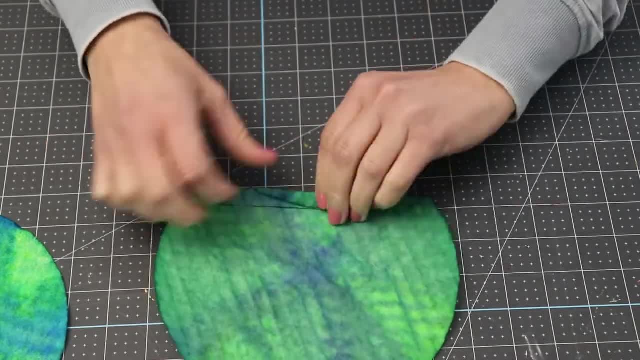 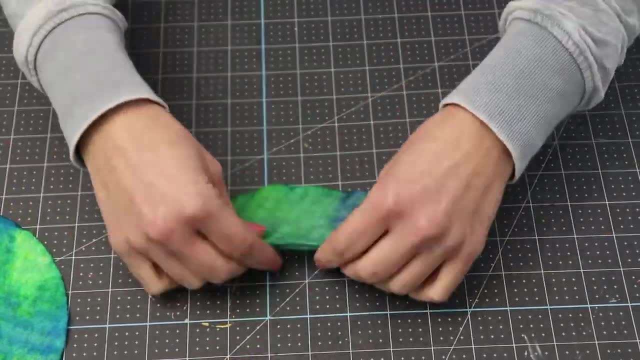 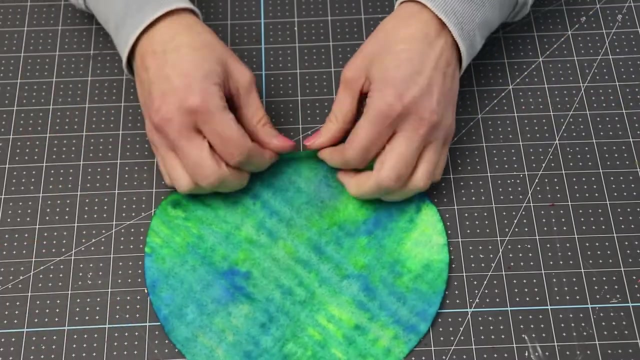 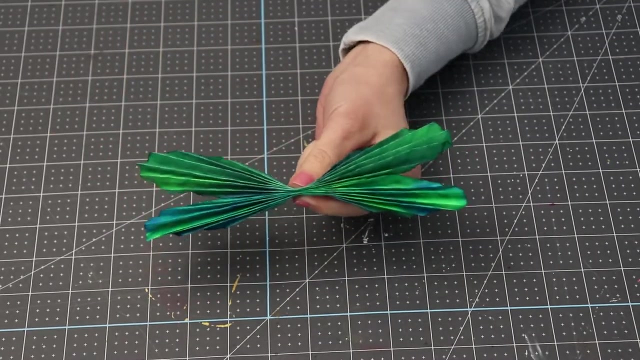 fold for each of these. Fold forward once, flip it over and fold backwards. Grab both coffee filters, press them together. These are going to form the wings of the butterfly. Then just wrap your pipe cleaner a couple times around the middle and form the two end pieces into little. 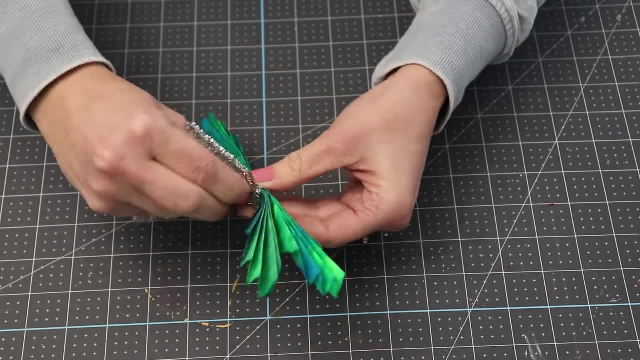 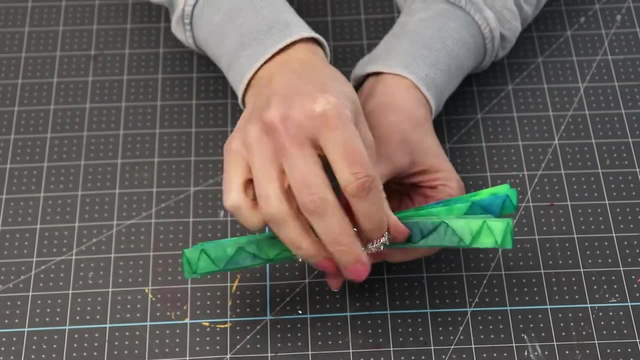 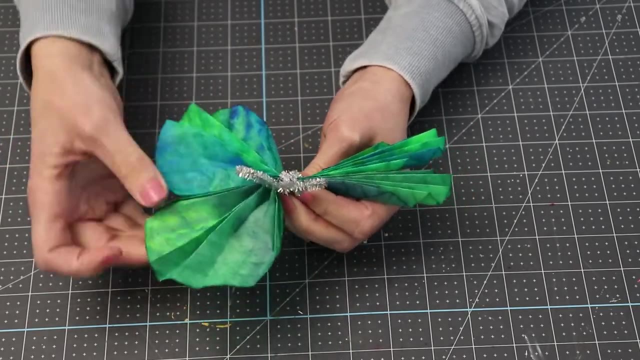 antenna on the top. there's no scissors, no glue. this is a really easy craft for kids. it's a way for them to get creative and get ready for spring. but I'll tell you, this is also a really fun craft for adults. I hope this inspired you to grab. 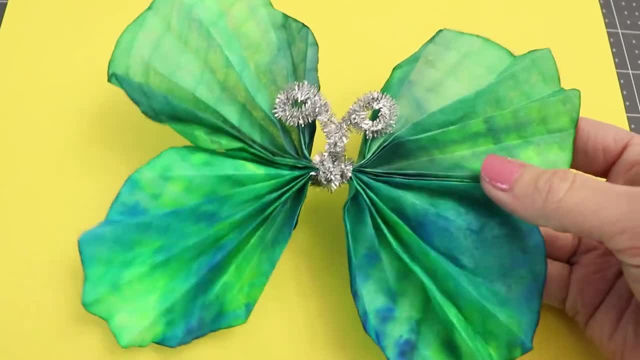 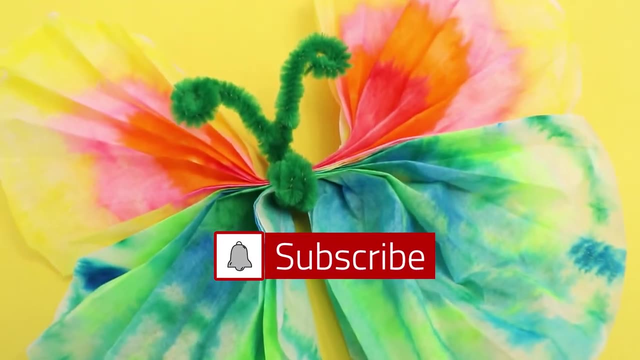 some coffee filters, markers, a little bit of water and a pipe cleaner to make these butterflies for spring. if you like simple crafts, hit that subscribe button. I am here every week with new simple craft ideas that you can try at home. thanks so much for watching. we'll see you next time.